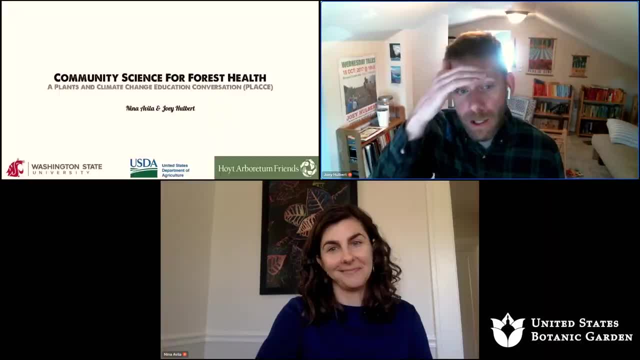 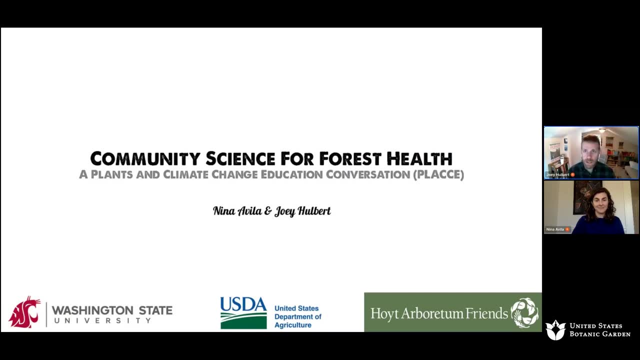 We're really pleased to be here. It's nice to be sharing this opportunity with Nina as well, And so I'm going to take the role first and share some kind of summaries of community science and how we're using it for forest health research. 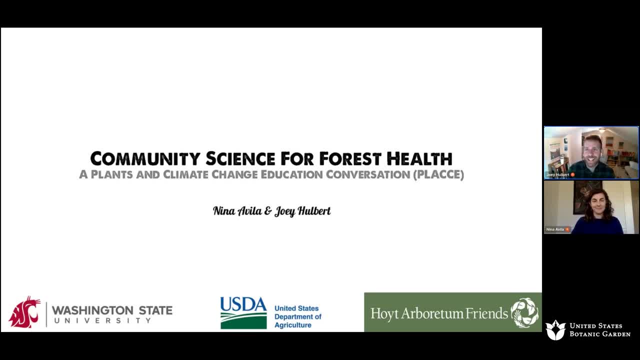 But I do want to welcome Nina, to say hello before we get started. Hi, Thanks for being here with me, Nina. Hi, Joey, Hey, everyone in APGA World, Thanks for joining us today. Yeah, Joey's going to get started and then I'll jump in in a little bit and tell you more about our project at Hoyt Arboretum. 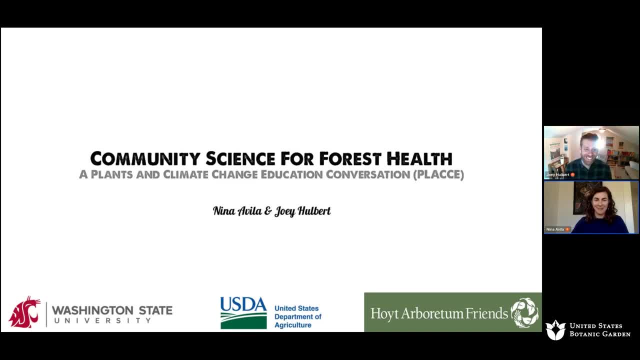 And apologies for my voice. I hope everyone can hear me, okay, This is not my normal sound. Thank you, Yeah, thanks, Nina. Okay, great, We do want to just kind of acknowledge where we're coming from and share with you today. 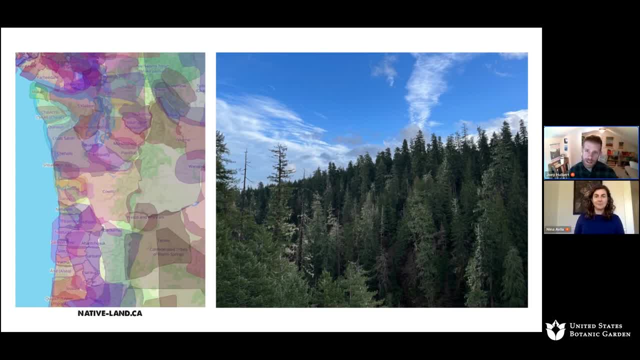 And I'm not entirely sure if you can see my mouse, Is that Probably not? huh, Yeah, Well, anyway, today I'm coming to you from the traditional homelands of the Puyallup tribe of Indians, Kind of in Tacoma, Washington, And Nina is joining us from Greater Portland area. 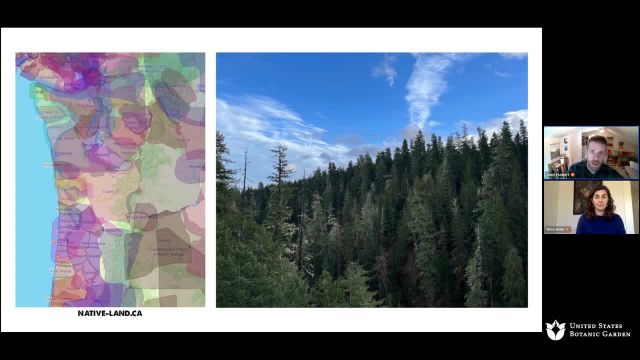 traditional homelands of the Calvets and the Clackamas and a couple other bands of like the Kalapuya, And we're just really pleased to be coming to you from kind of the lands of the Conifers and the great Northwest. 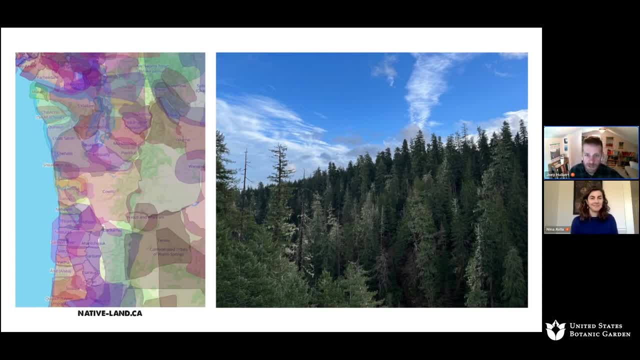 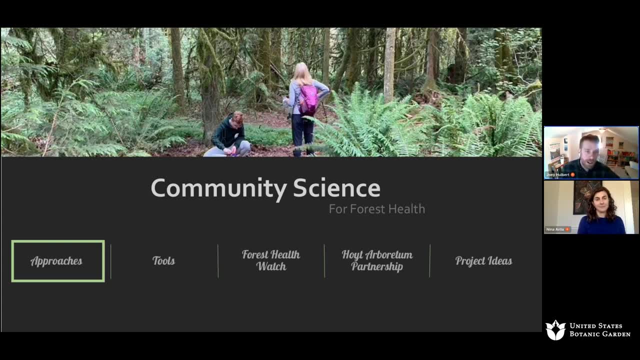 And we have had this extreme privilege to get to love and fall in love with the Northwest And we're thrilled to be able to share some of that love with you today. So, in terms of Community science, today we're going to highlight a few different approaches. 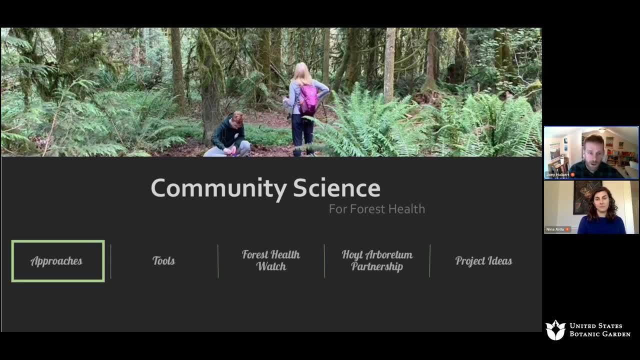 And what's really neat today is I'll talk a bit about one approach that we've been using, And then Nina will share another approach that we've been using to tackle kind of the same, the same issue in terms of forest health, And we'll introduce that soon. 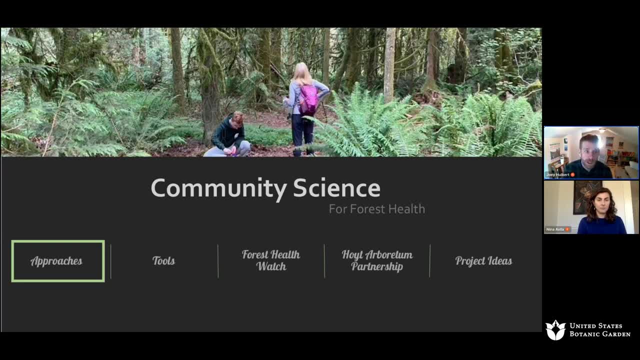 We also want to talk a bit about the different tools available for you to use in your garden if you're interested in engaging members of your community or volunteers, or or your own Staff and some of these research projects, And we'll introduce the Forest Health Watch projects kind of the research that we're collaborating with, Nina on. 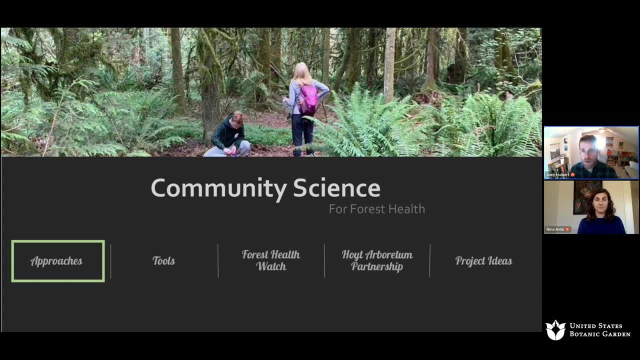 And she'll have some opportunity to share a bit about their programming at Hoyt Arboretum. And then we wanted to kind of wrap up with some summaries and some ideas of projects that could be done in other gardens and some places that we'd like to go together. 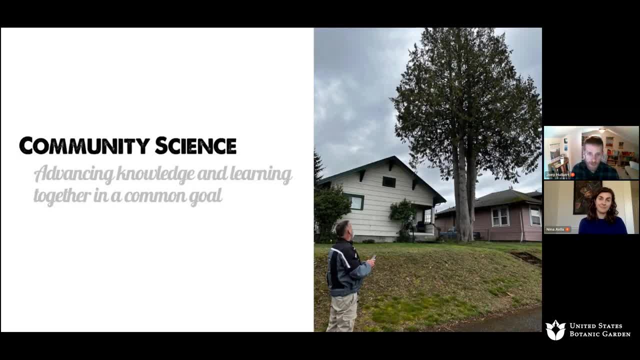 So pretty thrilled to be here. And this is a photo of an individual in Tacoma named Jim. He's an incredible community scientist in our in our program, And you know he he's been really one of the top kind of contributors. but he's also shared a lot with us and helped us shape other programs and other research questions. 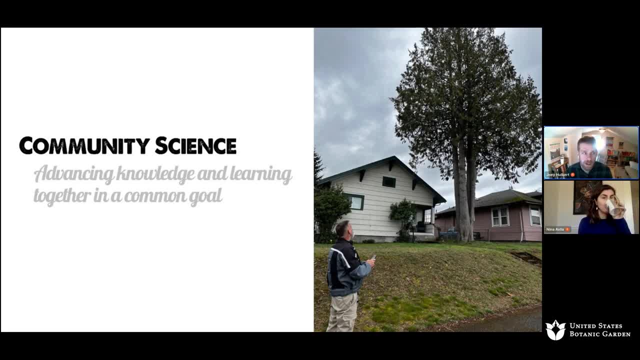 So in many ways we're we're advancing knowledge together, but we're also learning together, Like I'm learning from him, You know. I'd love to share with you some of the research projects that we've done, that he's basically brought to the table. 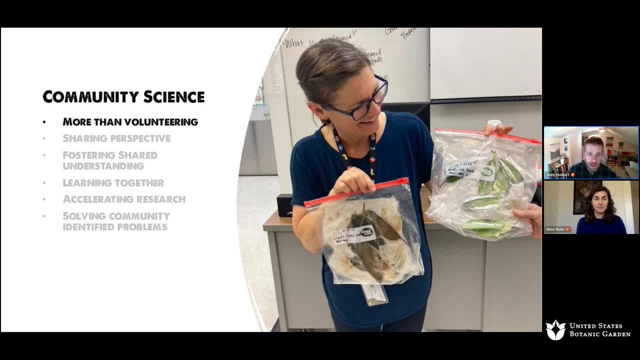 And with his own interest. But overall we think about community science as a lot more than volunteering. We're trying to build programing and opportunities where there's shared perspective. We want to build programing where we're creating shared understanding around certain issues and we're learning together. 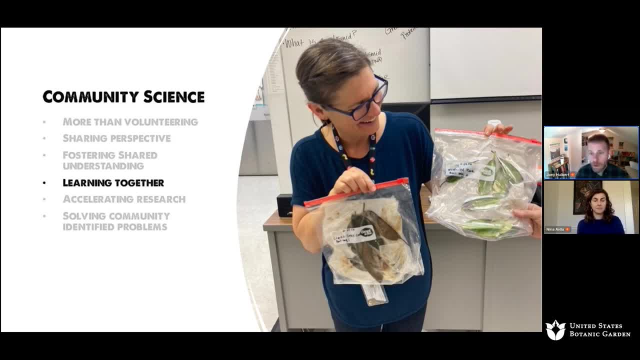 And so it's really a two way opportunity where we try to to build the programing in that way so that we're learning together and advancing knowledge at the same time. In some cases there may be a problem that you identify with the community. 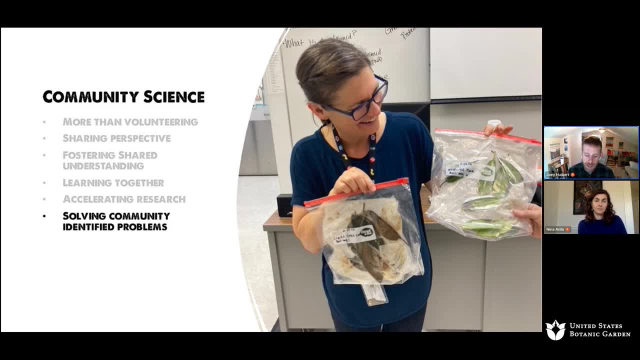 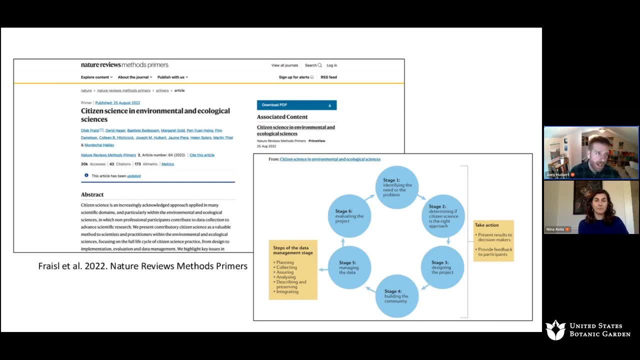 And I think, when that's the case, that tends to be the most powerful community science projects you can have, because there's a lot of intrinsic interest in the project to begin with, And I did want to highlight this- this study from Dr Frazel- that I had the super privilege. 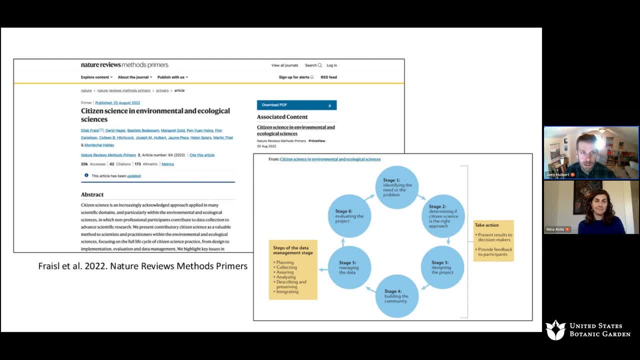 To be included on, But it's a really great paper in Nature Reviews that summarizes kind of citizen science or community science, if you will, in this role in ecological and environmental sciences, And I really like this diagram on the bottom right, where the first stage of this is what I just mentioned, where you identify a problem with the community. 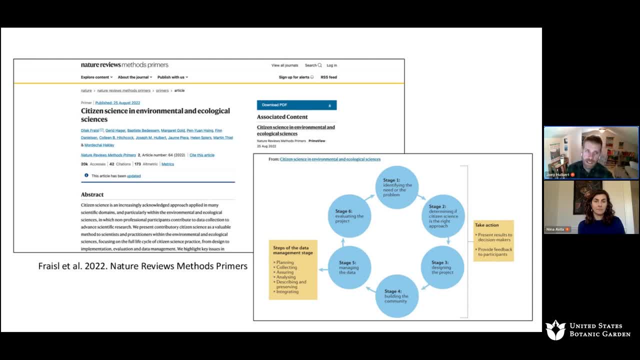 And then, when you have that problem in mind, you determine if citizen science is actually a feasible approach And from there, If So, then you, then you work to start designing the project and building community around it and collecting the data And then finally doing some evaluation. and today we're going to share with you a specific project in an issue in the Northwest. that's kind of 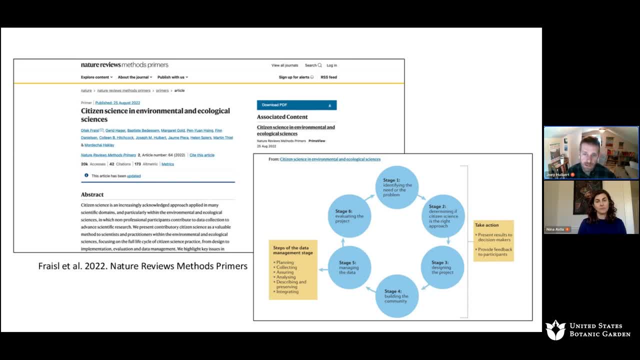 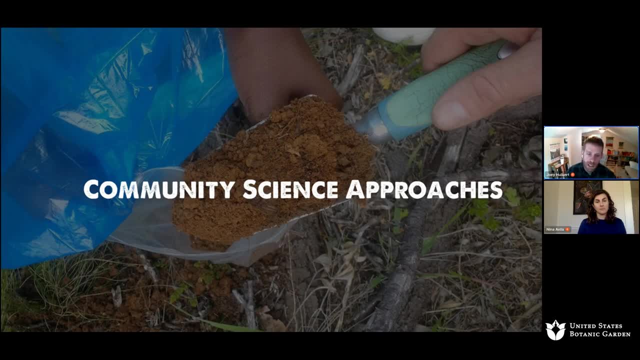 Kind of the reason we built this force health watch project and the reason it was the first project of the kind of broader program. So before we get to the specific project that Nina and I are Worked on together in the Northwest, we still want to just summarize kind of the different types of approaches you could use for building community science programming in the Northwest or, excuse me, in your garden. 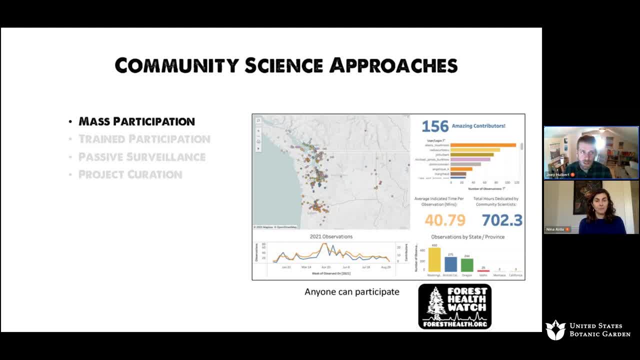 One approach is this, this, this type of approach which we consider like mass participation, where anyone can participate without any formal training, And this is this is great if you're trying to collect data over a broad scale, like we have in the Northwest, where we've kind of reached. 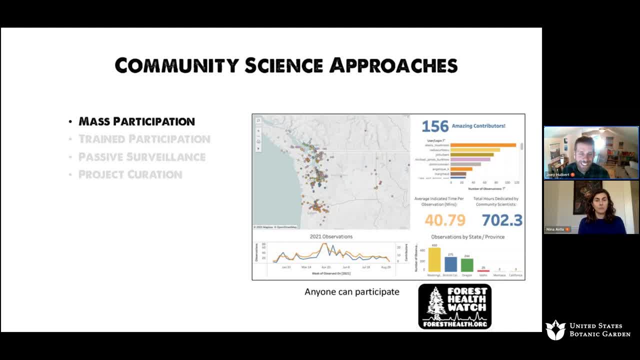 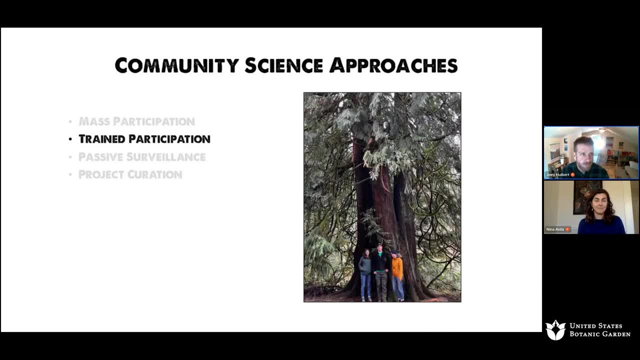 Communities. You know from ranging from our friends joining us today in Vancouver and Victoria all the way down to where Nina is in Portland. The other alternative that Nina is going to share a little bit about is this: more trained participation, and so in this case you're actually training a cohort of volunteers or participants there go through rigorous training. 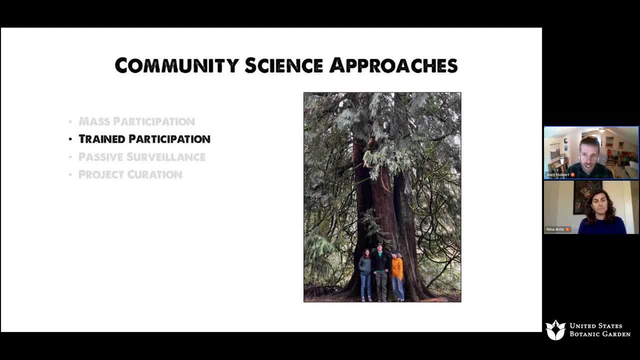 And then those that cohort is the team That's collecting the data. it's not really open to everyone, but you can do a lot more powerful research in that way sometimes. for example, Nina will share with you kind of how we engage some volunteers in an actual hypothesis test. 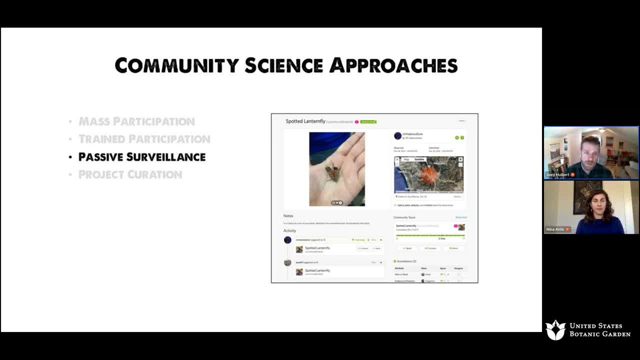 Using that method, Another approach. Sometimes I refer to it as passive surveillance, but it's really like by the biodiversity monitoring. So in this case it's a observation on I naturalist, Where someone shared an invasive insect and they may not have known it was an invasive insect. 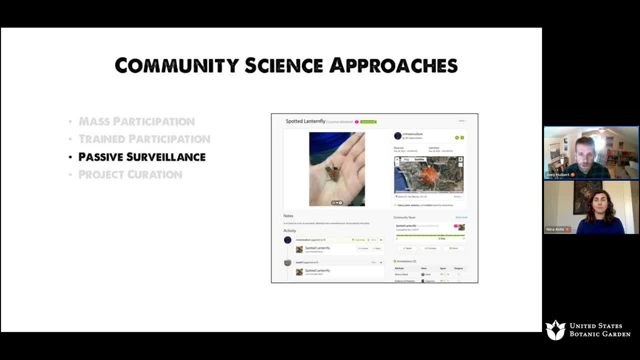 But in that case, you know it's an opportunity to kind of surveil what's happening and what people are seeing In nature and in, or their, their own cities or your gardens. you know you might find the first spotted land to fly in California. 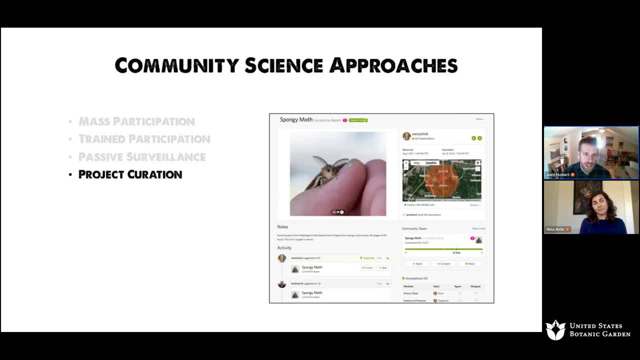 On. I naturalist, you don't know Until you start looking. This other approach is a Little bit different in. This is kind of an approach for where you may set it up. so individuals are contributing to project curation or enhancing data quality on some of these tools and so 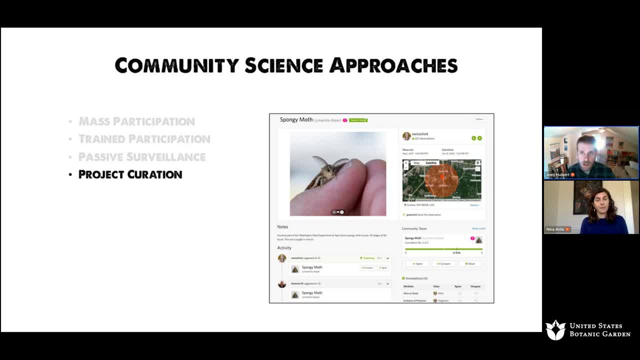 Again, this is I naturalist, which I'm going to talk about in a minute when we get into the tools. but there's one of the powerful things about this is the community. in here there's a ton of dedicated individuals that help in help people identify. 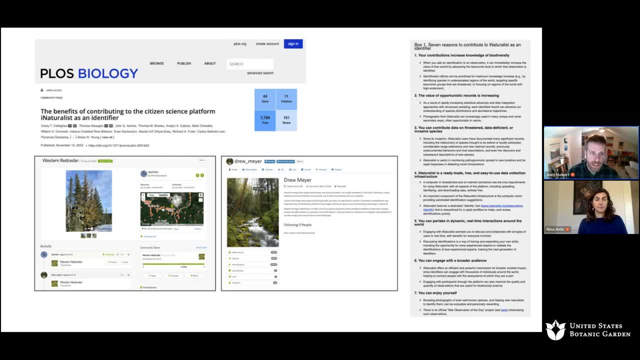 Organisms they add, and so I want to share this example of Drew Meyer. so he's a kind of an amateur, I think you know he had. he sort of identifies as a birder but really is just passionate about all biodiversity, and he has identified more than 67,000 observations on I naturalist. 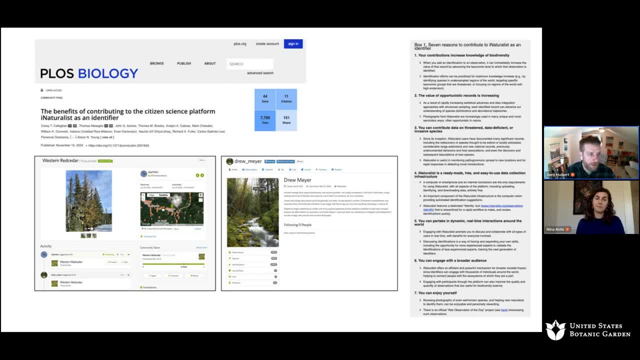 So it's kind of just this unsung hero and I'm really, really I'm grateful for individuals like Drew, because they really help us maintain the quality of data that's shared. in some of these tools, like I naturalist, where it takes multiple people to agree that they identified that we're going to correctly. 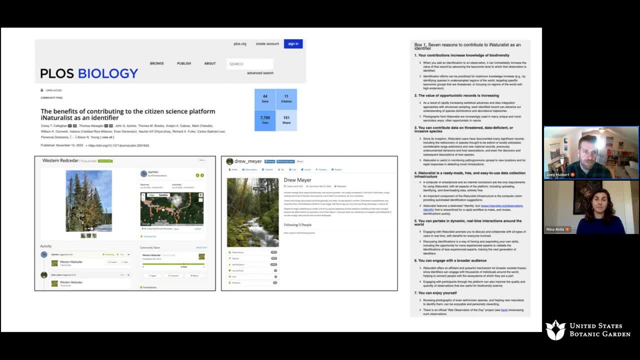 And I like this paper that kind of summarizes the benefits of, of that approach, of engaging as a community scientists in that way. You know they highlight a lot, of, a lot of great value that you can add to just from your own computer. But this one might be especially valuable to us in this community. 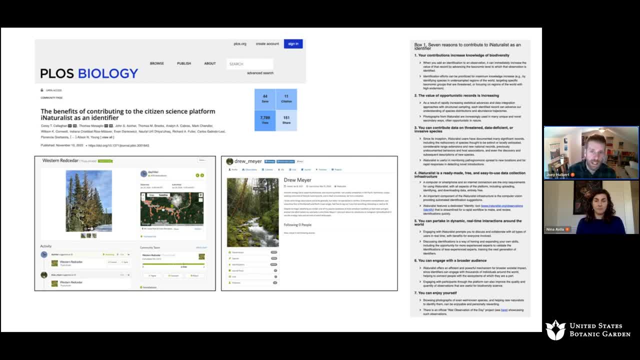 Now you can contribute to data on threatened or rare data, deficient or invasive species, You know, without having to be there in person, and you can engage with broader people. You know there's just lots of good that you can do, and so you may be thinking like well, we have this volunteer base. this would have been really great activity. 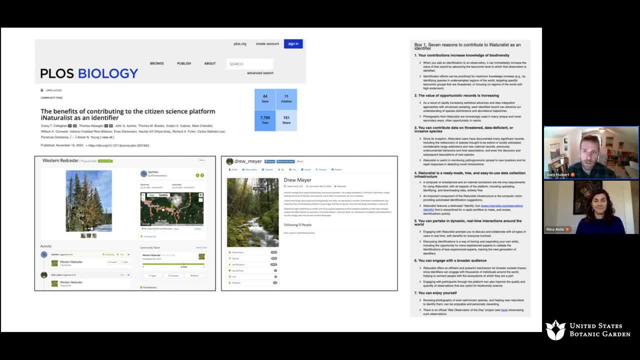 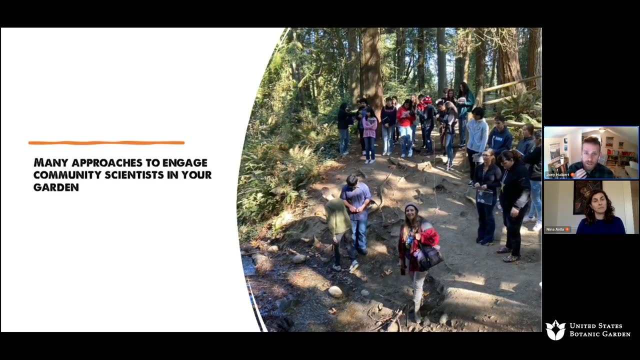 During cove it or from from some remote land learning standpoint, where you could come together online and then work together to a debt, you know, to help the community around you identify some of the biodiversity. But overall there's a lot of different approaches. you know we talked about the trained approach or the mass participation. there's a lot of different ways that you could be engaging more people in your own gardens. 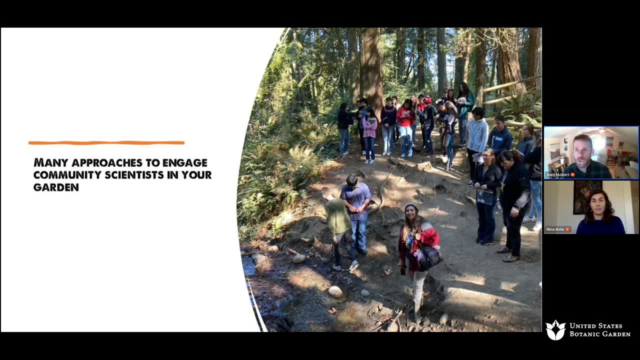 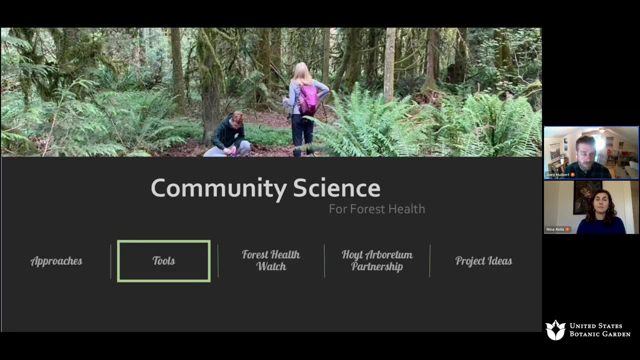 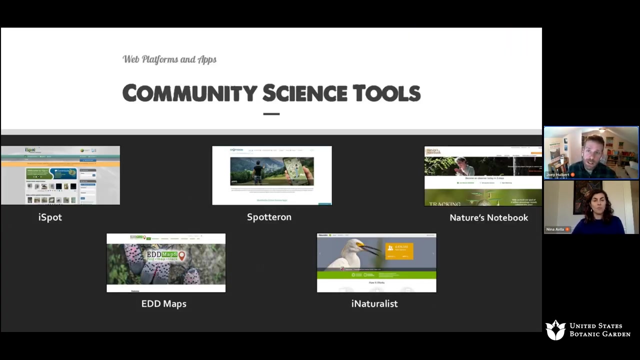 To think more critically About what they're seeing into, to Add some observations to broader research projects and things like that. The next thing i'm going to highlight is just some different tools that you could be using. so we just talked a lot about I naturalist and i'm going to talk a bit more about it, but there's a number of other tools. so nature's notebook is a really incredible tool and, specifically, if you're interested in 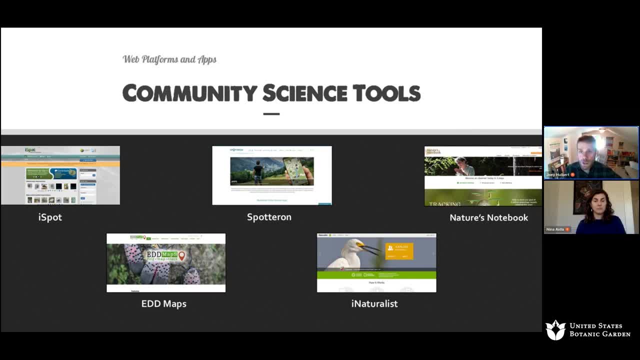 Climate change Type of phenology work where you're looking at the timing of blood bursts or something like that. there's there's a lot of great projects within nature's notebook, kind of focused on. that spotter on is another another kind of mapping similar to ED maps. you know, mapping is biodiversity and same with I spot. they're all kind of different in the way that they. 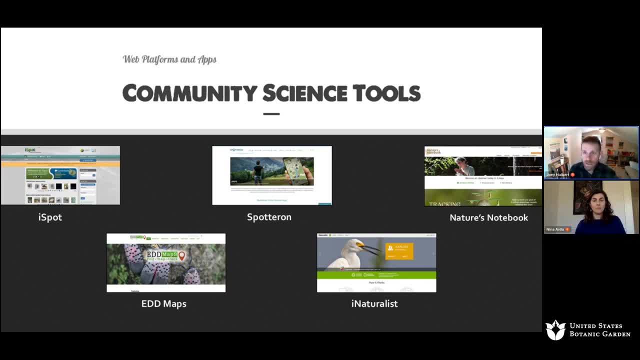 They work with the Community. I spot allows you to have like symbiotic relationship, so you're tagging multiple organisms in a single picture, kind of, and you can, you know, link this pollinator to that flower, for example, and so each of these tools have their own kind of benefits and and drawbacks. but 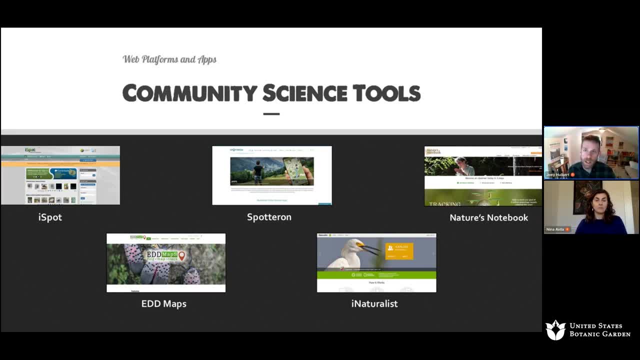 The other thing to think about is the Community that you're in and what tool that Community is using the most. so we can talk more about that, but I did want to just spend a couple minutes Telling You why. for us, we really like a naturalist. 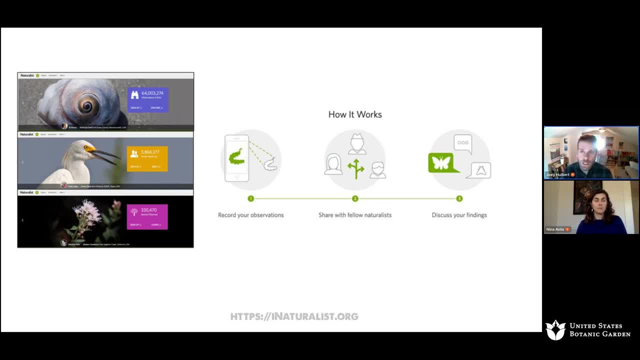 Generally we pick a naturalist because it has a pretty good user base and really we liked it because the data is all open and available to anyone. We also liked it because it has a really stable smartphone application, so we don't have to worry about updates every time your phone gets a new software, new. 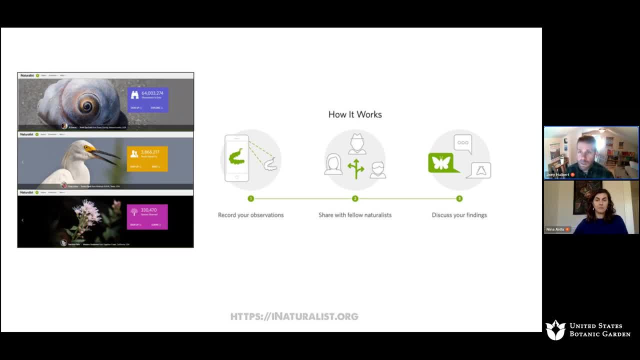 You know Every time your phone updates. but the way it typically works is you just take photos with your phone And you shared on a naturalist and other people will help you confirm or deny whether you correctly identified that organism and once you kind of have a Community consensus, it's considered a research great. 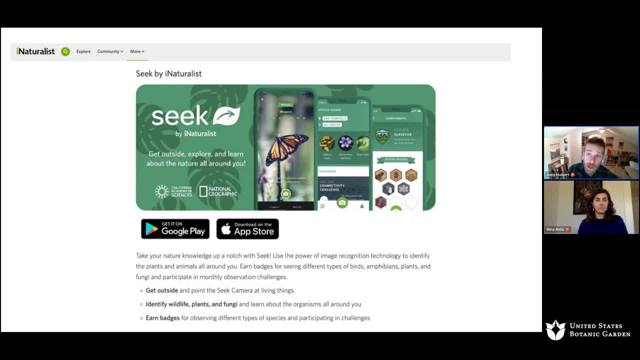 Within this, we've effectively trained a computer to identify things with photos now as well. so I naturalist created another APP called seek, which is super powerful and really useful for identifying biodiversity, and so you just hold your camera up to a plant or an insect and it will throw you some suggestions based on the models that has been able to train with that Community feedback. so it's pretty cool to see that you know you're not only just contributing to research and biodiversity monitoring, but you're also helping train 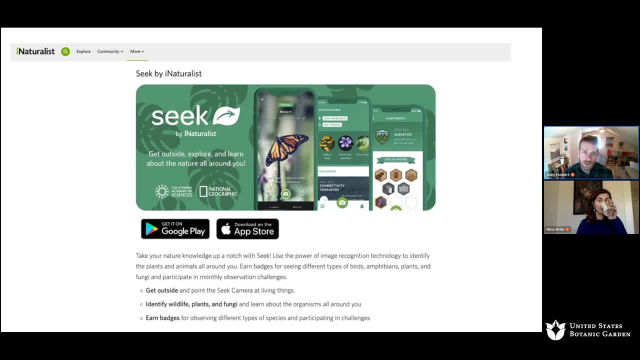 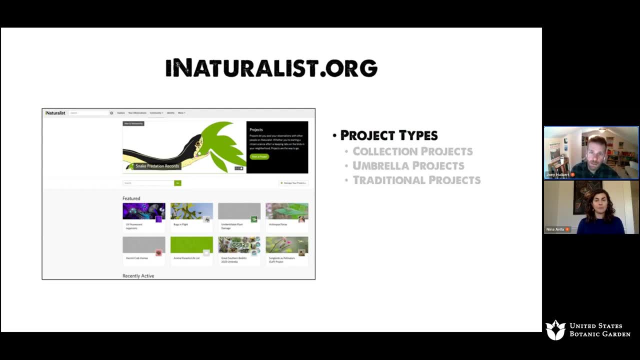 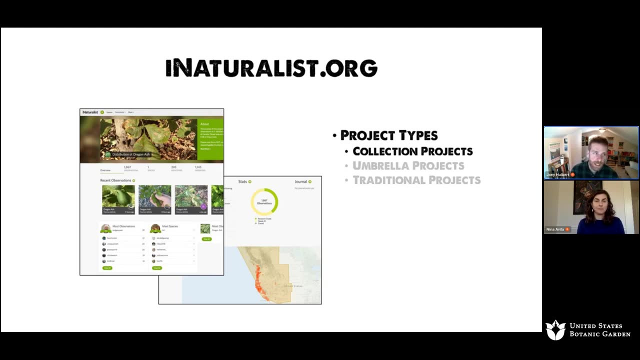 You know, A tool that could be used In your garden as well. Within I naturalist, there's a lot of flexibility. there's a couple different project types. The most simplified is this collection project, and so, in this case, I have 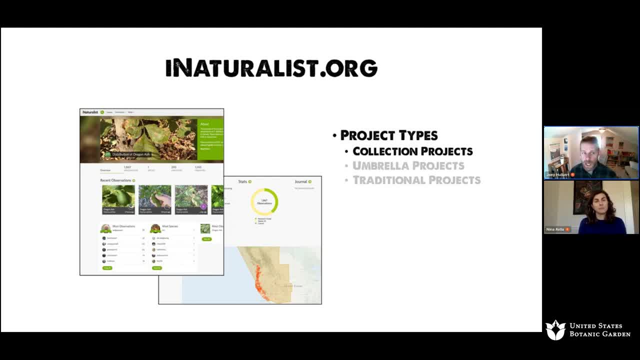 i've just said, I want you to collect every observation of Oregon ash within the western us. you know automatically creates a project with all the observations of Oregon Ash and so you could create A space for your garden, you for your arboretum in this and you could say biodiversity of white arboretum and you draw the boundary of Hawaii arboretum and it automatically will collect all the observation shared with a way arboretum in one collection project. it's pretty neat. 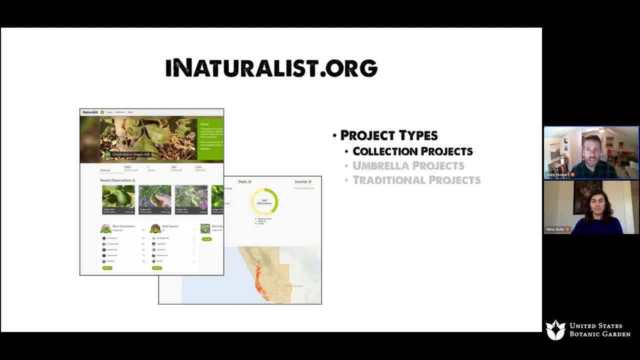 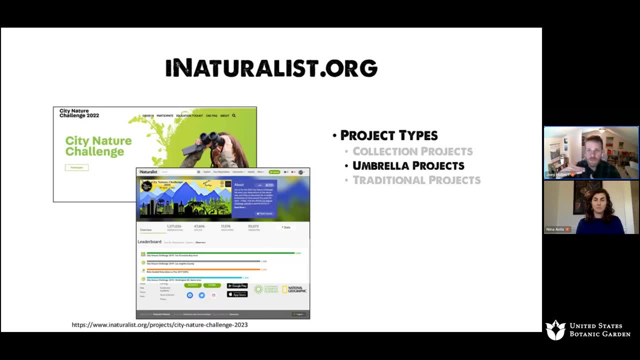 And then with that you could do some even cooler stuff where you're competing or you're sharing or you're comparing with other gardens. So there's these umbrella projects that take multiple collection projects And allow you to compare Different metrics like number of participants, number of observations, different species observed, and so the city nature challenge is a perfect example of that, where every year, 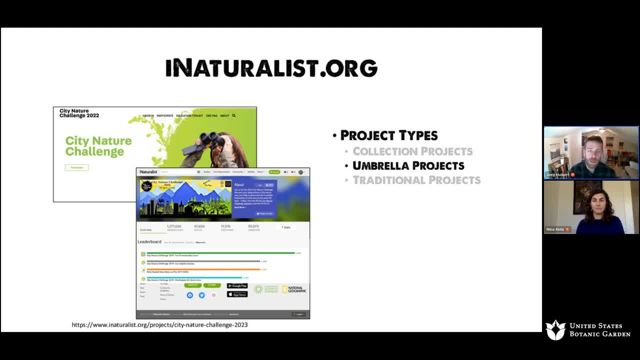 Between- I think it's the last week, so April- and the first couple days of May, they do a bio blitz, ground the globe and they ask individuals to add observations of any organism within that one weekend. then you're kind of As a city, you're kind of competing with other cities throughout the world to see who can document. 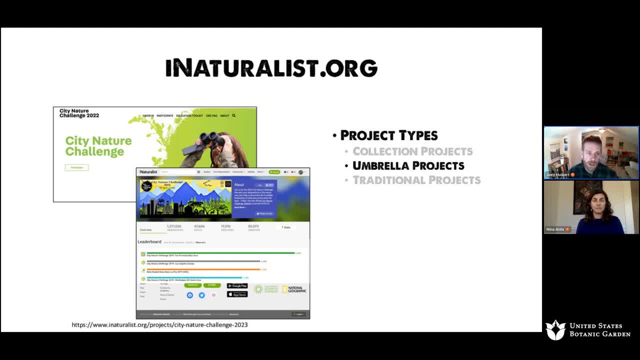 the most biodiversity in that one weekend, and so it'd be really fun to do that with all the gardens on this call. right, if we had kind of hey, during this week we're going to try and engage all of our communities to map biodiversity and then we want to compare which gardens have the most. 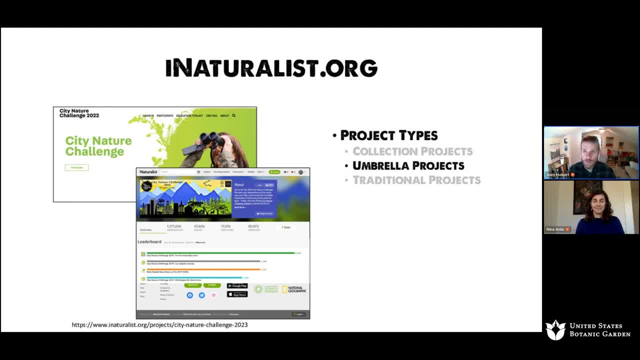 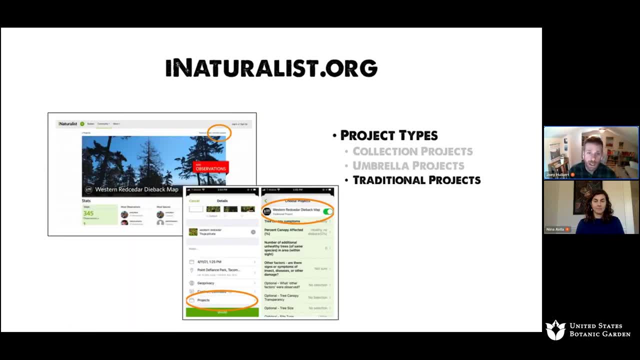 biodiversity or you know, just compare, like kind of you know, the different species in different gardens or there's a lot of neat things that you could do depending on what your own interests are. the third project type in iNaturalist is this project type called traditional. they're the 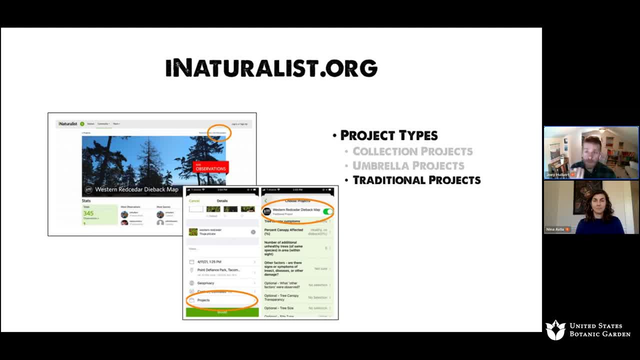 traditional projects and these are custom. they're like, very customizable. you can create all the questions in the project and so in this case we created one about a tree disease or tree dieback issue in the northwest, this western red cedar tree. that i'll talk a bit about more in a minute. but the way we did this is you. you would. 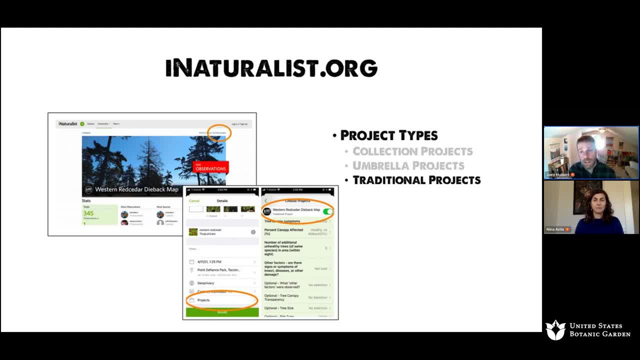 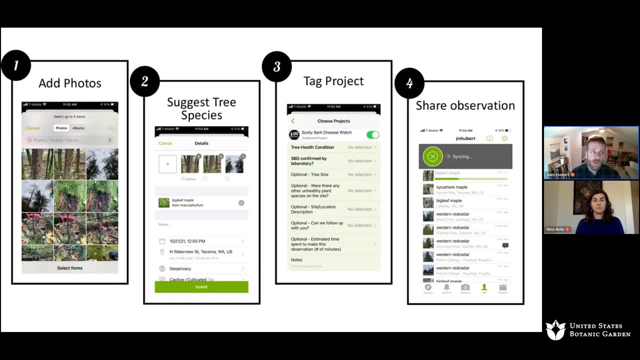 join the project and then when you add a observation of a red cedar to the project, it asks certain questions like: is this tree a healthy tree or an unhealthy tree, is this tree next to a road or is it in the middle of a forest? those kind of questions. so the way this works is you would add pictures. 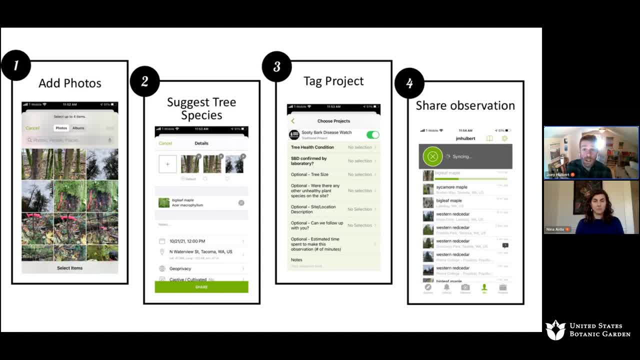 in your garden on your phone with iNaturalist or your computer. you can also take pictures with your camera and then later add them via your browser, your internet browser. but it's certainly easy once you've done it a couple times on your phone. so you just add a couple of photos. you suggest an identification for that. 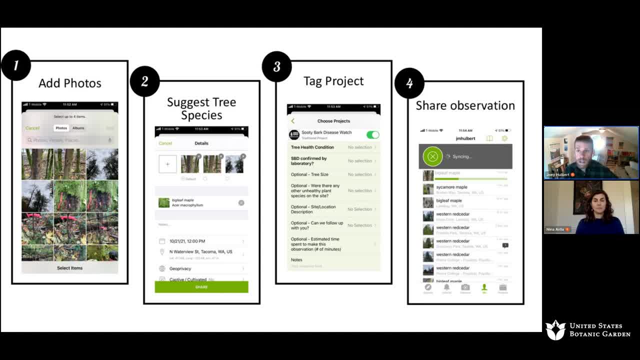 species. so in this case i'm adding some big leaf maples, but these, this case we're adding a maple that has a disease called sooty bark disease, so i'm adding it to my garden and then i'm adding it to this project. so i tag a project and when i do that it asks me all these questions. 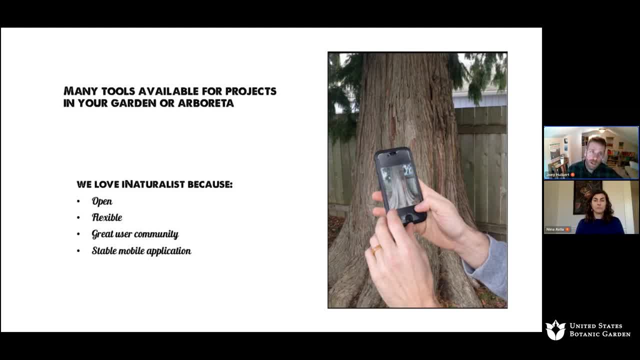 so, in summary, there's a lot of different tools. you know, really, they're all. they're open, they're available, they'd probably love to support you and work with you to integrate it into your garden and your community. each one has a little bit different benefits and stability and things like that. 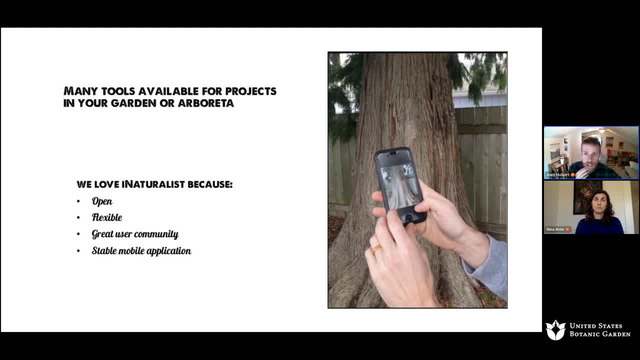 but really something to think about is like: what is the community around you already using? but generally we love iNaturalist because it's open, it's flexible, it's all those custom, you know, all those project types. it's got a great user community. it's very positive. there's lots of people already using it and we know that it's. 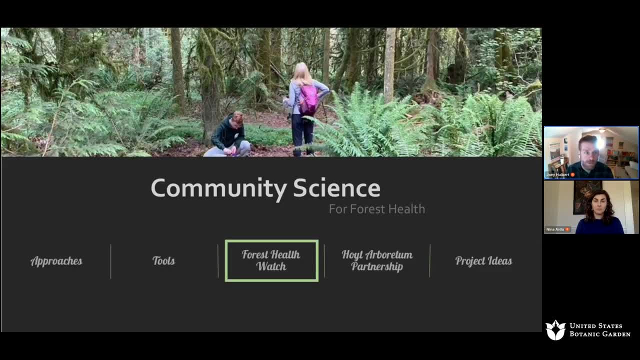 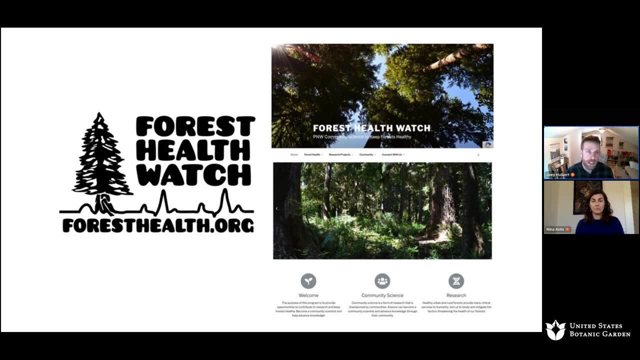 going to last into the future. it's like really stable. so with iNaturalist, we've been focused on a tree health issue in the forest health watch and, as we mentioned previously, we created this in 2020 with support from the USDA. we still have some funding from the USDA to maintain this project. 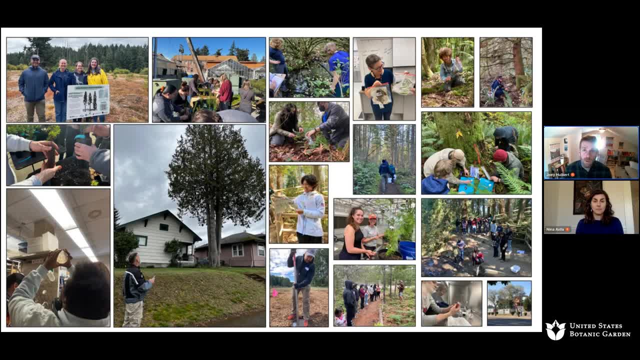 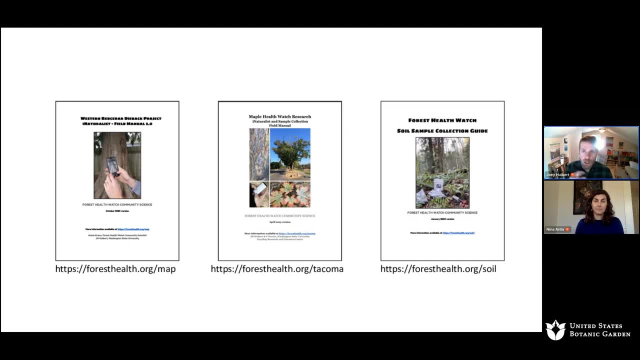 it's been really grateful for that support, but we're even more grateful for the many community scientists that have helped shape this program and make it into something meaningful and useful. so within the forest health watch we've kind of done, we've kind of worked on three different projects so far and i'm really just going to 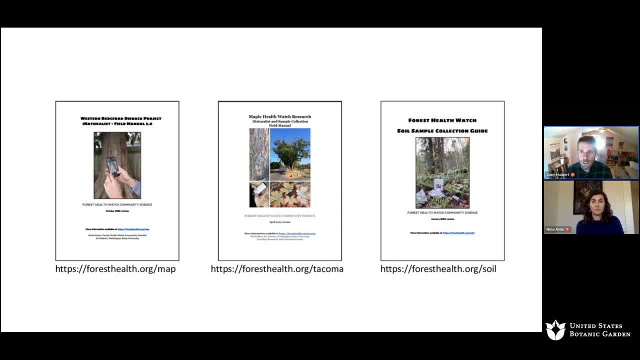 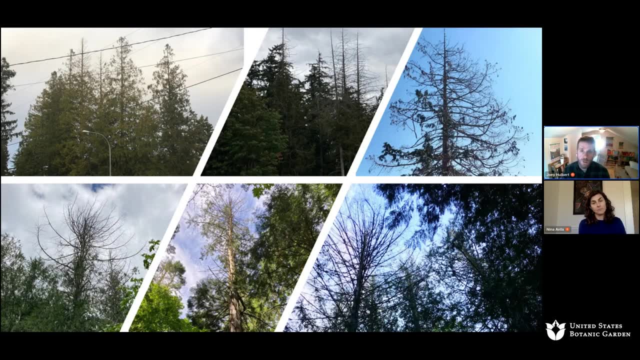 highlight this first one today, which is really focused on western red cedar and using iNaturalist to map the health of red cedar in the northwest. so, unfortunately, we've been seeing a lot of dieback in the species, which is at least on the west side of the state where i am and where nina is. it's characterized by these top, the tops of the. 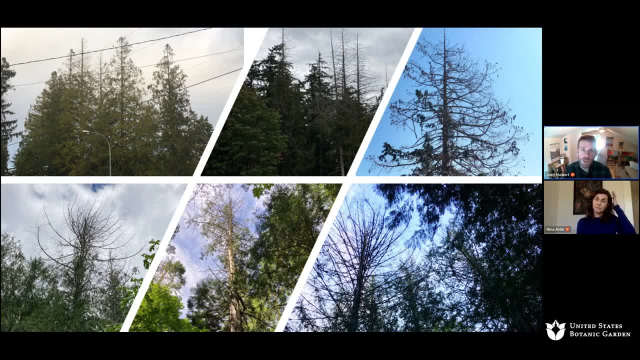 tree dying. it's characterized by these tops of the tree dying. it's characterized by these tops of the tree dying, and many times that leads to complete mortality, and so, unfortunately, we see this throughout the range and there's been some questions about. you know what is driving this, but there's also been 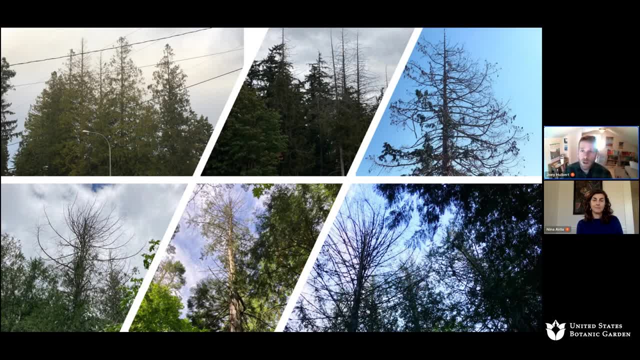 some answers, but initially, when we started, we asked our stakeholders and partners: what should we focus on? what should we engage communities in? what's some? you know what's the greatest concern? and western red cedar dieback was the biggest concern for all of our partners. so it's the first. 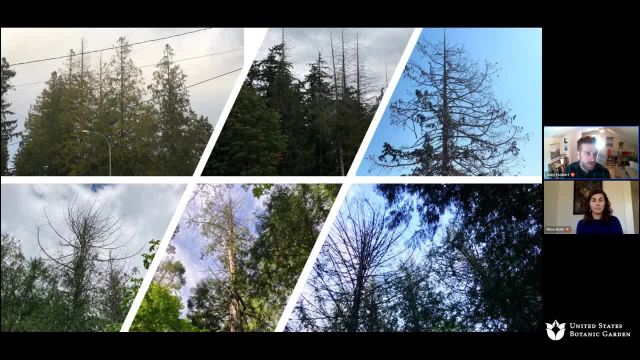 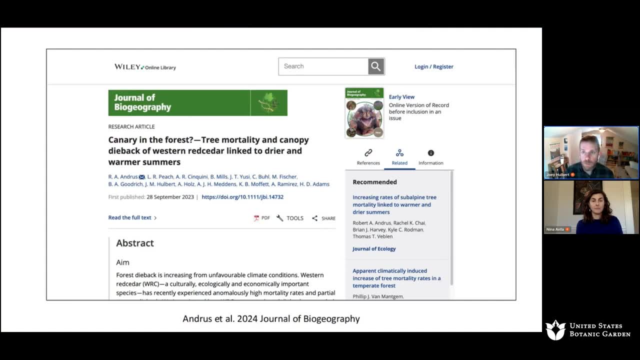 project we we launched in the forest health watch. since then- this is from just this year- a colleague of mine did a nice dendro dendro chronology study where they cored trees and they looked at tree ring growth in relation to climate, in relation to drought, stress, and they 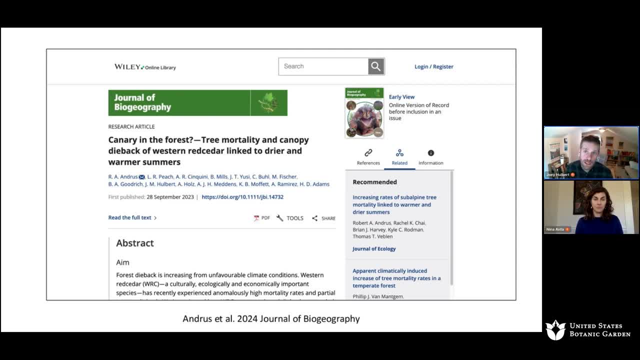 found. you know this. this dieback issue is largely driven by consecutive longer and hotter summer, and that's kind of an issue that the northwest of the us is faced with, because we're used to having droughts, but they seem to be getting longer and hotter, um and so, depending on where you are, 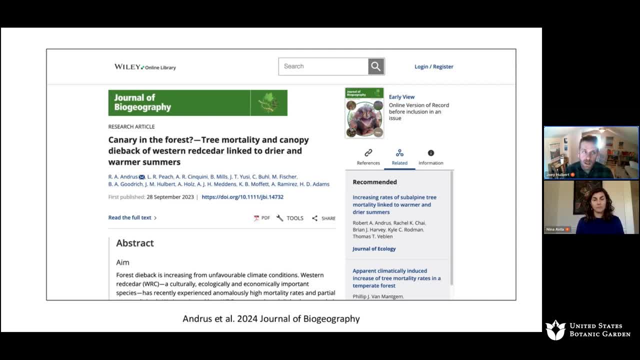 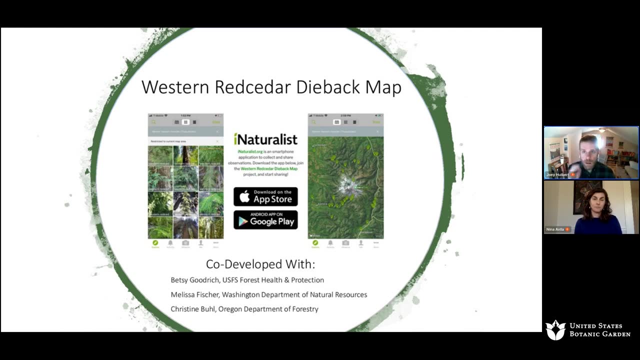 you know, that signal might look a little different. but now that we know that red cedar is likely feeling the heat of of these droughts, there's a lot of opportunity to kind of explore some specific hypotheses and and dive into that deeper. so after in 2020, when we first, just you know, decided this is the focus, we 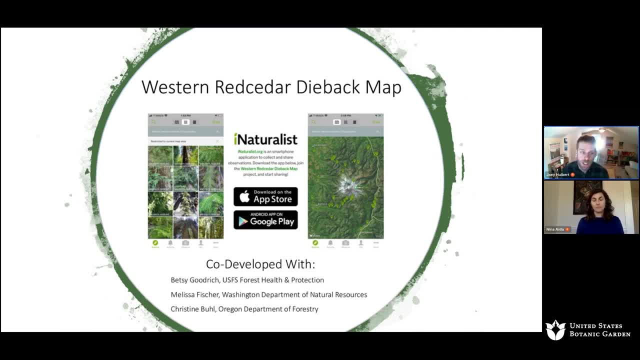 are really grateful to work with a number of partners from state agencies and federal agencies to design this high naturalist project. so these three individuals were really generous and they were already kind of tracking this in their own agencies and they worked with us to create this high naturalist project that's open to the public but also asked the same kind of 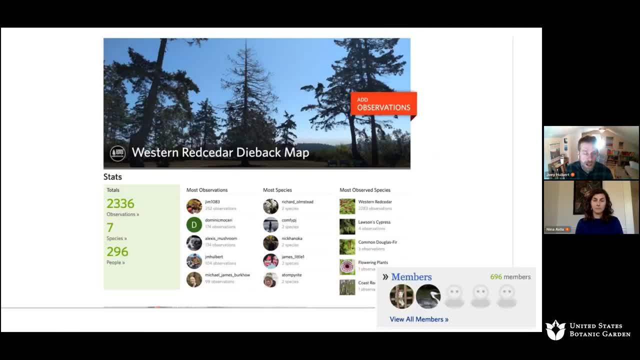 questions that they're asking and they're looking for, and this is um a little bit, maybe a couple months old, but so far we've had around 300 people share observations, but almost about 700 people have joined this project and are interested in it and we do. what's another thing that's neat about? 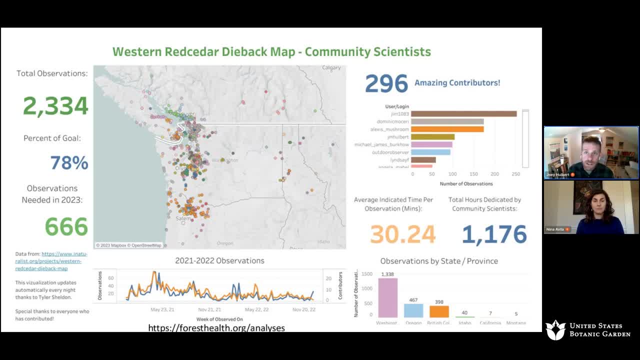 inaturalist is you can take this open data and you can integrate it into other software or other apps and you can use it to create a dashboard and tablo public, and so there's some neat ways to kind of see this update every day, and this is available on our website, foresthealthorg. 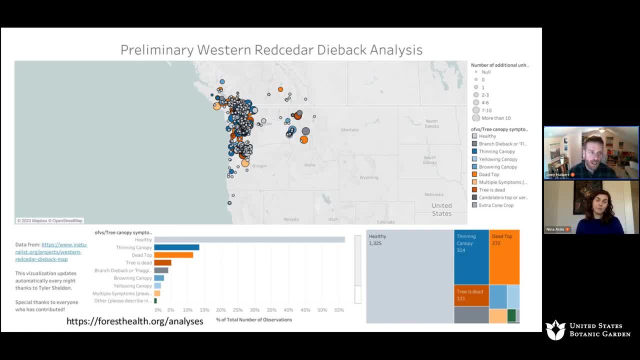 similarly, we created one with the health metrics and so you can kind of click on these and see where all the trees have been shared and where all the unhealthy trees have been shared. so these are all the trees with dead tops right. so similar to that photo i showed you. 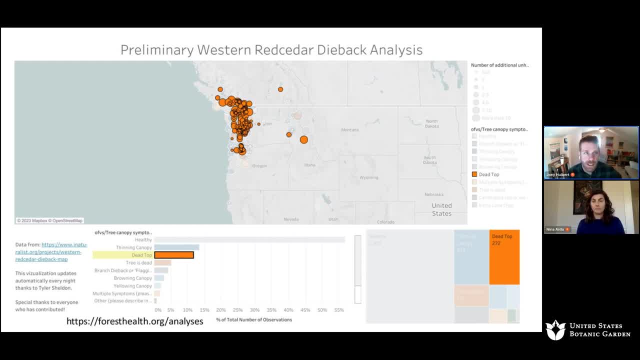 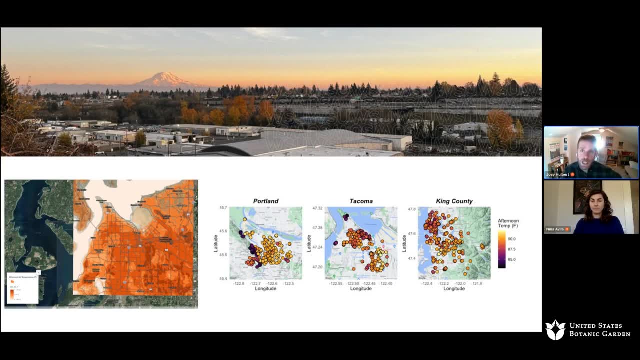 those series of photos. we're seeing this die back throughout the range. more recently, with with nina's help, and something that we're really excited about at the moment is we've started to look at the red cedar trees from that data set, from the inaturalist data set. 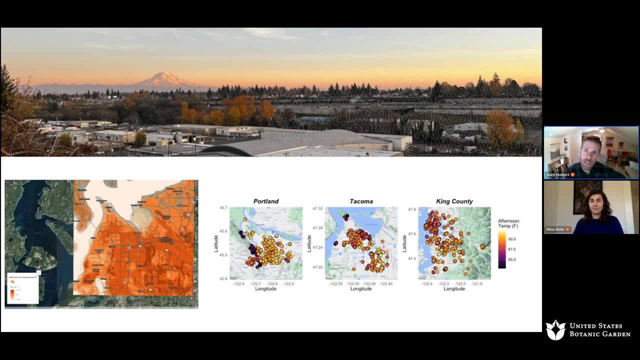 that are in the urban areas and we're interested in testing a hypothesis about the link with urban heat. and so between seattle and tacoma- this photo is tacoma and portland- there's these great heat maps from urban air temperature mapping campaigns and we're able to extract that data and explore. 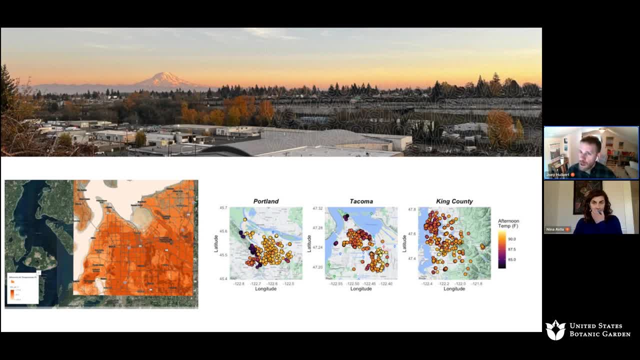 you know this hypothesis of whether, um, like, we hypothesize that the trees in the hotter areas and heat islands are going to be less healthy than trees in the cooler areas, and this has been a really fun opportunity to work with nina and her team to explore this hypothesis. and then the the capacity to leverage community science to 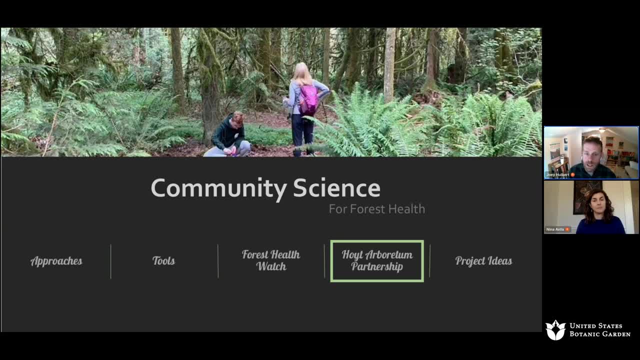 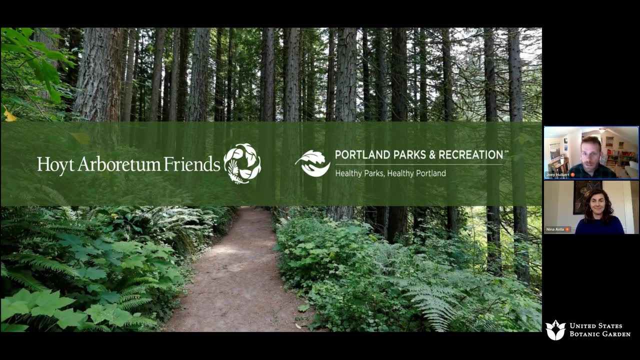 address these, these questions, and so at this stage, we're going to hear from nina on what that looks like from white arboretum's um perspective. so go ahead, nina. i hope i left. thanks so much, joey um. thanks for giving us a great introduction and overview of community. 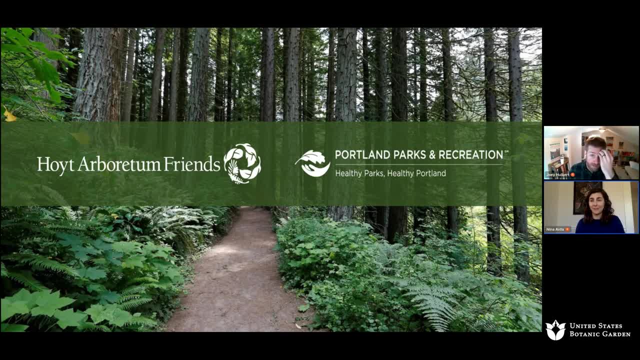 science, um, and how the forest health watch is making a difference up here in the northwest, um. so hi everybody. my name is nina aguila and i'm the education programs director for white arboretum. friends, um, i want to tell you a little bit about a white arboretum. 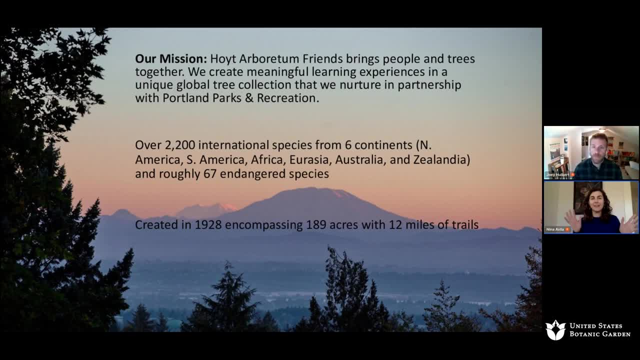 first, just to give you a little background information. um, so you can picture it, we are a space of about 189 acres. we became an arboretum in 1928 and we have 12 miles of hiking streets of 189 acres. and we became an arboretum in 1928 and we have 12 miles of hiking streets. 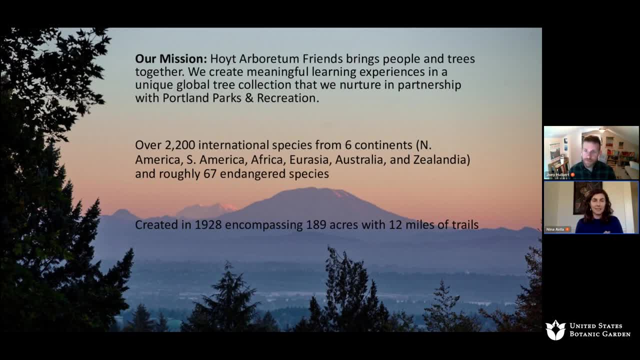 trails. So along your hiking trails you'll find over 2,200 different species of trees from six different continents across the United States- I mean across the world. We have a global tree collection and 67 of those are endangered species. So I work for Hoyt Arboretum Friends and we're 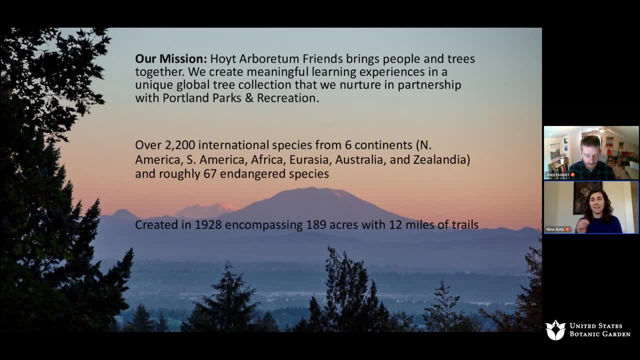 the non-profit that brings trees and people together. We do a lot of the people-y things at Hoyt Arboretum. We manage the volunteer services, we manage our visitor center, we have a membership program and we have lots of great education programs. So we do the people-y stuff. 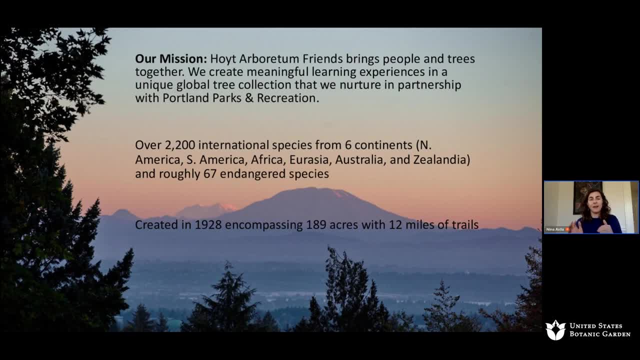 and we work in partnership with Portland Parks and Recreation to take care of the tree collection and the trails, And we're a free, open park. this is it's a little different than a lot of you out there that might be at a botanical garden that has an admission. We're free. we're open all the time. 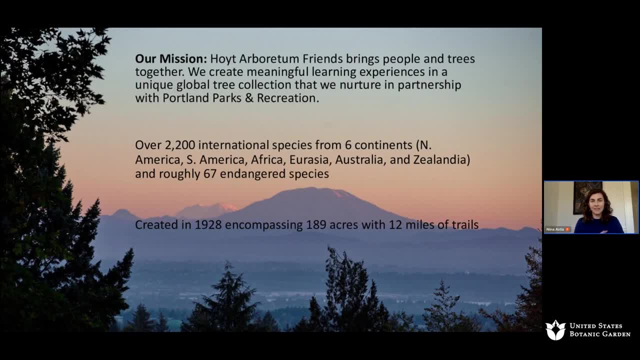 so we're open. We get lots and lots of visitors at our space and this is a really this is one of our clear days in Portland. The picture behind the words. you can see a picture of St Helens and I believe that's Rainier in the background behind it. So we do have clear days in Portland. Today's actually a beautiful. 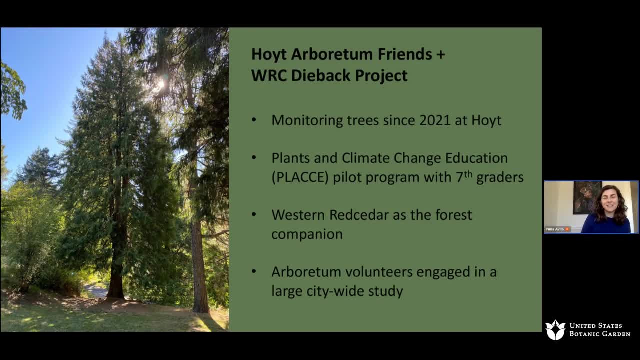 clear day. So how did Hoyt Arboretum and Joey and the Western Red Cedar die back? How did we get together? Well, in 2021, there was a group of dedicated volunteers at the Arboretum that were like Joey said. they were part of this cohort that was trained. They were trained with staff at the 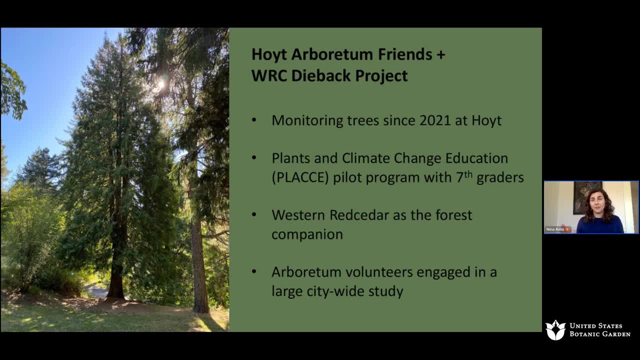 Arboretum and with Joey on the Western Red Cedar dieback project, So really understanding what's happening to the trees and what does that look like. And then what they were doing was monitoring the trees just at Hoyt Arboretum on our property, so within the 189 acres. 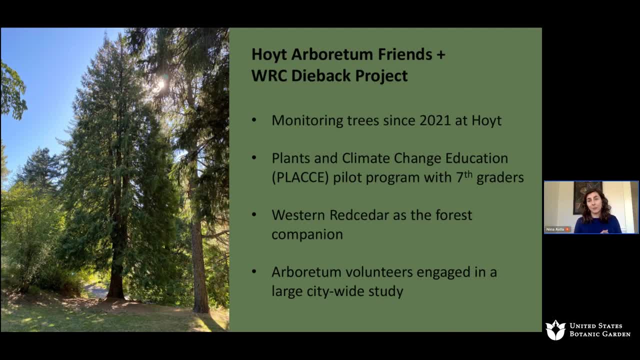 And they've been doing that on an annual basis since 2021. And that's a picture of one of my favorite Western Red Cedars at the Arboretum. Yeah, and then in 2022, like as Emily introduced we are, we became part of the the place program, the cohort Hi to all of my cohort friends out there. 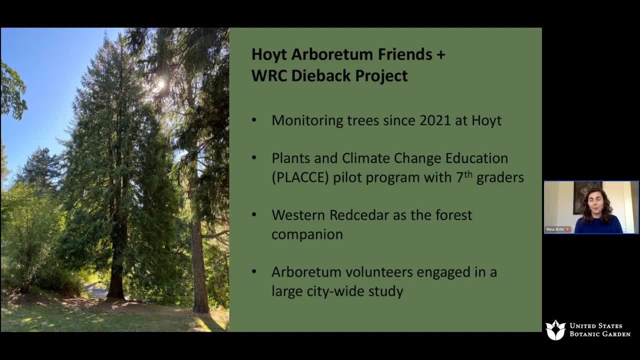 We had an opportunity to submit a proposal and my particular proposal was about middle school schoolers and climate change education. There was a gap in our programming at the Arboretum in middle school education and it was also. I was understanding that it's kind of a great time to. 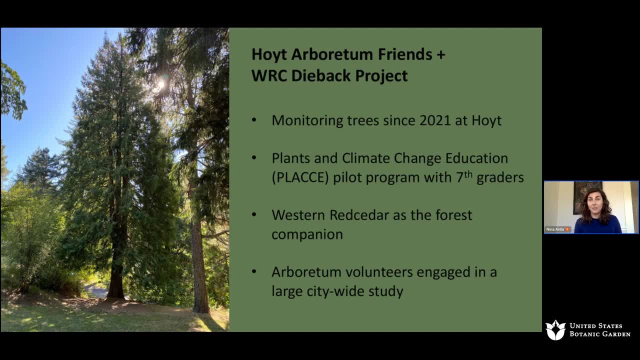 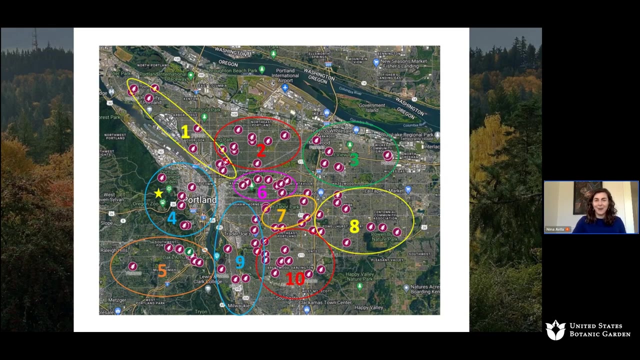 really start talking to students about climate change, and what better way to do that than with plants and trees? But we needed to have a focus and if you're ready for a tree, pun. a tremendous connection was made: The Arboretum. oh, let me go back. The Arboretum chose the Western. 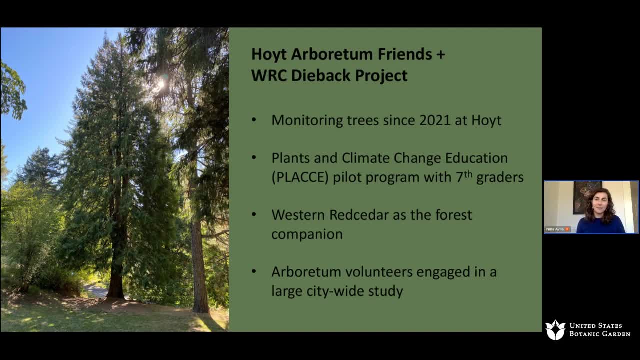 Red Cedar as the forest companion, with as a focus with the middle school students. So Joey and I started talking. I needed to learn more about his project and Western Red Cedars And through our conversations this big question came up that he mentioned earlier. 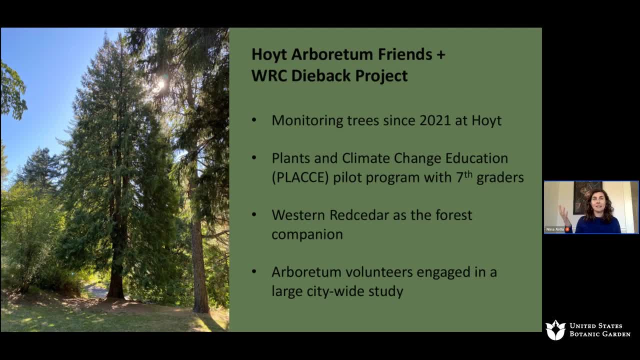 Is there a correlation between Western Red Cedar tree health and hotter spots and the temperatures in Portland? cooler areas, hotter areas- Where are we seeing a decline in Western Red Cedar tree health? So Joey was like: hey, can you get some volunteers to help us? We need more tree observations. So I said yes, which I tend to do before, If you know. 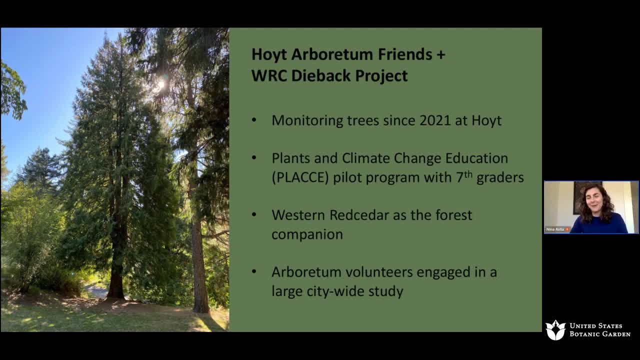 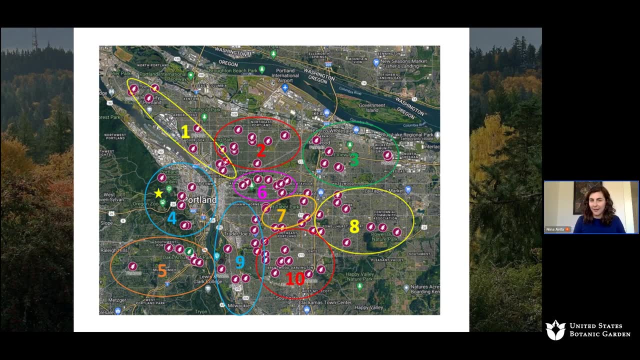 me. I say yes a lot and then I try to figure things out afterwards. So that's what I did. We said yes and Joey used the street tree inventory for Portland Oregon. It's available. Portland Parks and Recreation has made this inventory and he was able to select 100 Western Red Cedar trees. 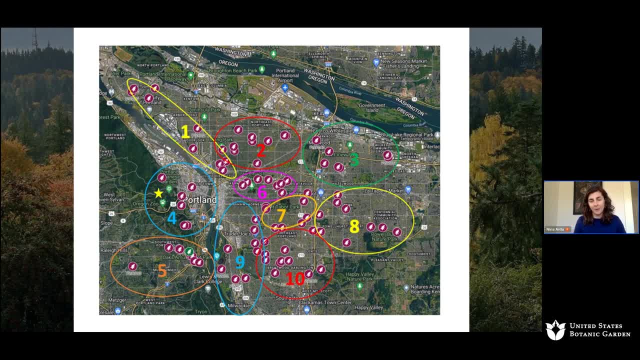 with a 30 to 40 foot DBH or diameter breast height throughout Portland. So what we did to make this kind of easier to digest for all of our volunteers is we grouped it together in like 9 or 10 trees, So we had this complicated map and then we had seven dedicated volunteers and myself and 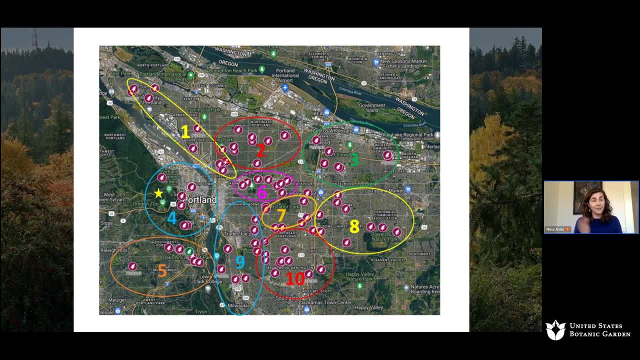 a co-worker And we went out and in the fall of last year we made all these tree observations using inaturalist as our platform. So, like Joey showed earlier, we all had our phones. we were out there. we were able to select the Western Red Cedar diebag project when we were. making our observations and answer the questions that correlated to that offset that we had on the platform that we were looking at for the February booster tutorабend. So it was really all in the column that we were looking at. And then one day when I went into the bag, Joey said: Oh, I'm not. 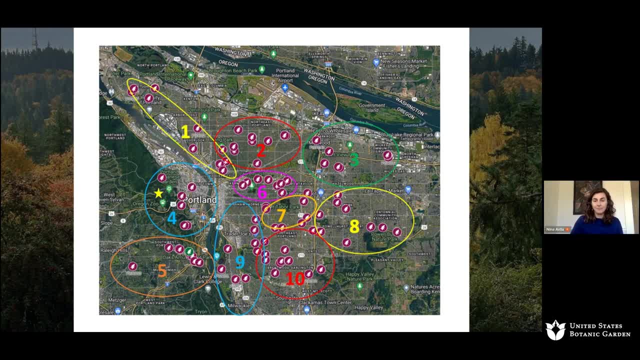 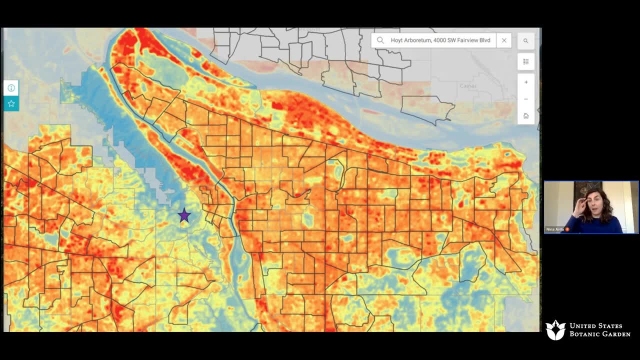 to the health of the western red cedars. So Joey was able to see all of our observations and then he was also able to take a heat map of Portland. So I just wanted to give you an overview of what that looks like. So I don't have a pointer, but the purple star. 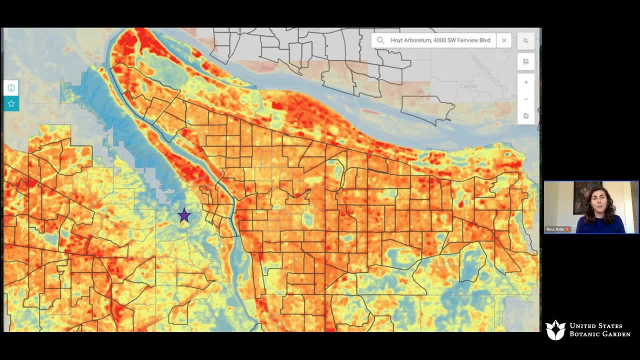 is where Hoyt Arboretum is located, and Portland is divided by a river called the Willamette River. So you'll see that blue line kind of going north and south and that divides the city into an east side and a west side. So Hoyt Arboretum is the star. We're on the west side of Portland. 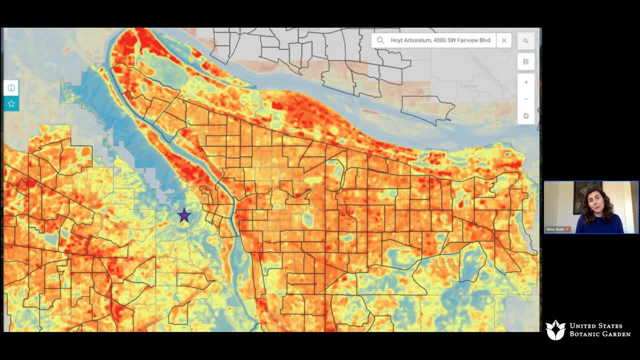 and we're in an area of blue. Blue means cooler temperatures. We are lucky enough to also be adjacent to Forest Park, which is like the largest urban park in the United States, and you can see where the tree canopy cover really makes a difference with Arboretum and Forest Park. 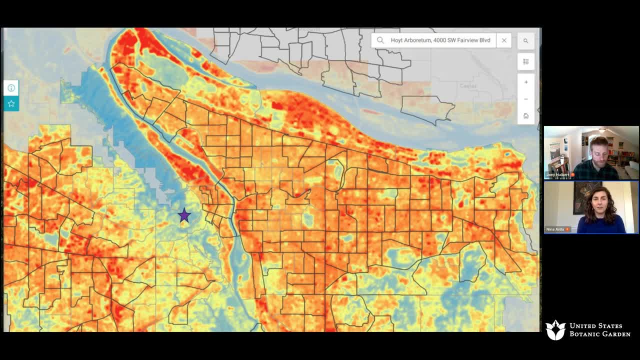 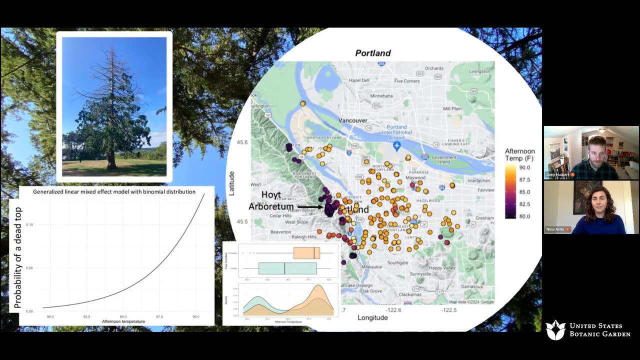 The area is. excuse me, the areas that are really red are the hotter areas of Portland and you can see they're kind of next to where the rivers are, that industrial area and a lot of eastern east side. Portland has increased temperatures So Joey ran some statistical magic, So it remains to be you. know. one thing we want to do now is like: okay, what can we do to keep these big trees healthy When we know they're vulnerable to heat and drought? right, what are some things? And we have just a couple minutes left, so I will kind of end with a final question. Maybe both of you can respond to you giving us such cool examples of community science work that you've been engaged with. When we do this and when we engage volunteers, we learn so much and there's so many more. they have great ideas. So you know, I think we're really interested in this Red Cedar story and I mentioned Jim. early on. and he, he, this past spring was like, hey, I want to know if the trees that have more browning right now um are the trees that had less water. we try and do stuff that has, you know, community needs um, so we're trying to assess. you know what is the next big question? um, what is the next issue that we should be aware of? and, um, and you know, is it feasible to to do anything meaningful towards that with community science? um, but, yeah, I think there's a lot of questions. um, within the red cedar, you know, we know it's. vulnerable now. how can we help it? what can we do for our big, large trees right now? is there something that we should be doing in Hoyt to make sure that they stay nice and big and healthy? um, and then too, you know, if we're going to replant red cedar because it's so culturally important. uh, can we plant trees from further south, um? or, you know, can we breed some drought tolerant um version of red cedar, I'm not sure like those. those are kind of next steps with that species. yeah, we'd also love to do a seed collection project where, yeah, where, we leverage the community scientists to collect seed and then we can store the seed and conserve that genetics um or grow that tree if it's a good candidate for for replanting other places. yeah, yeah, thanks, Joey. how about you, Nina, any thoughts on um future, future hosts for how you might like? to engage with community science and the work that you do. yeah, I think um Joey's always got a lot of great ideas, so, um, well, I think what I'm most excited about and can see in the future is- I hope there's one of our students that like asks a really powerful question this spring. and maybe that leads us into a different direction for next year. um, we're hoping to continue our, our pilot project from place. we're hoping to continue it into the coming school years. um, but yeah, maybe it's not always western red cedar focus. maybe there's another question. that's coming up, or I'd love students to be more engaged in their, like, local school neighborhoods, getting teachers involved, making it more part of their curriculum. so I'd really love to just keep engaging students and teachers and seeing, seeing where it goes kind of organically, but, um, yeah, but. the western red cedar. like Joey said too, there's a lot more to go from there. um, from where we're at right now, yeah, thanks, lots of possibilities and yeah, the more we learn, the more questions we have, of course. so, always, always, do things to explore, um, I want to say thank you so much. to both of you for joining us this afternoon and thank you to our participants who came and and had such great questions and really engaged with us throughout this program. thanks so much for being here.